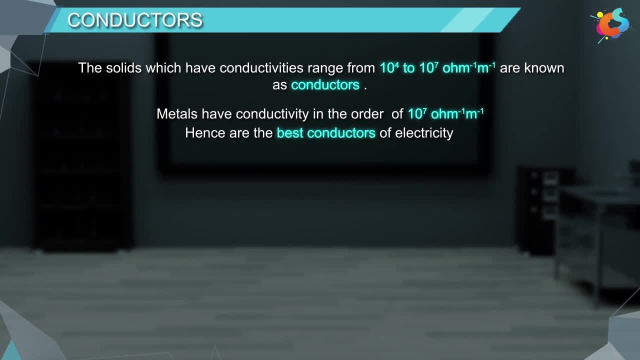 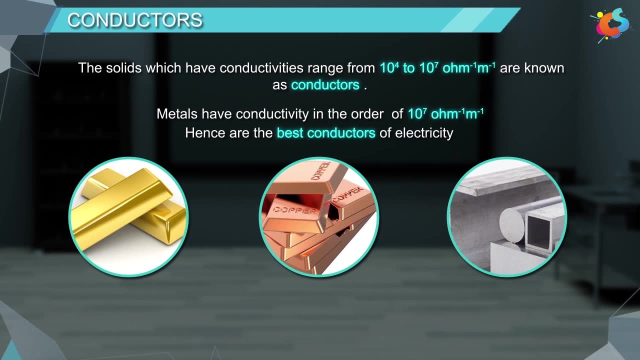 Conduction of electricity in metals. Metals like gold, copper, aluminium, etc. are very good conductor of electricity. They can conduct electricity both in solid and molten form. The extent of conductivity in solids depend upon number of valence electrons. In metals the valence band is partially filled. 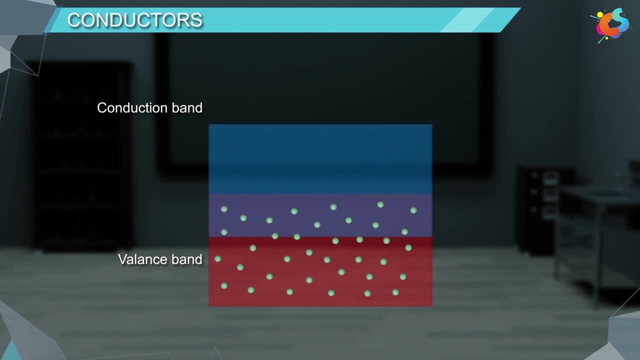 And usually only a small amount of valence is filled. The valence band overlaps with the empty conduction band in such a way that there is no forbidden gap present. As a result, the electrons from the valence band can easily move to the conduction band. 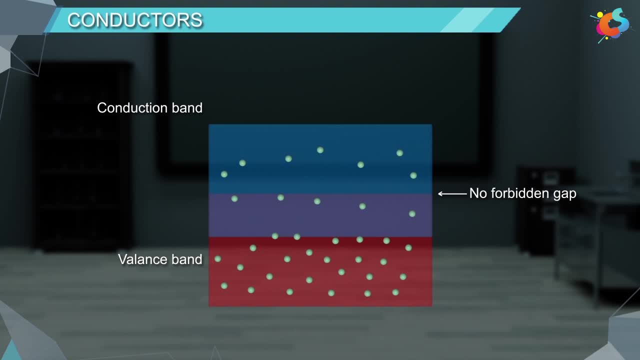 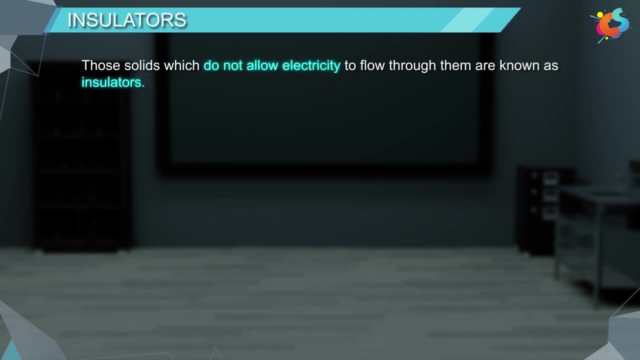 This results in conductivity in metals Insulators- Those solids which do not allow electricity to flow through them, are known as insulators. Conduction of electricity in non-metals. Conduction of electricity in non-metals. Nonmetals, like plastic rubber, do not conduct electricity. 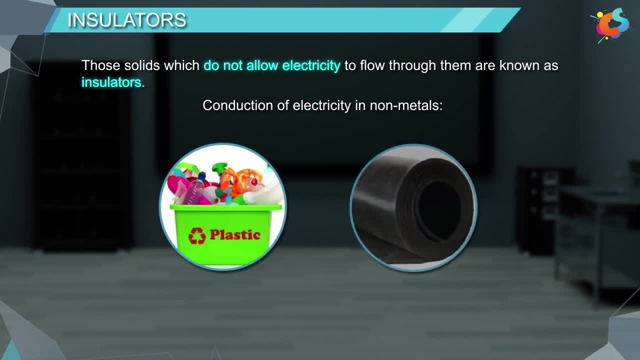 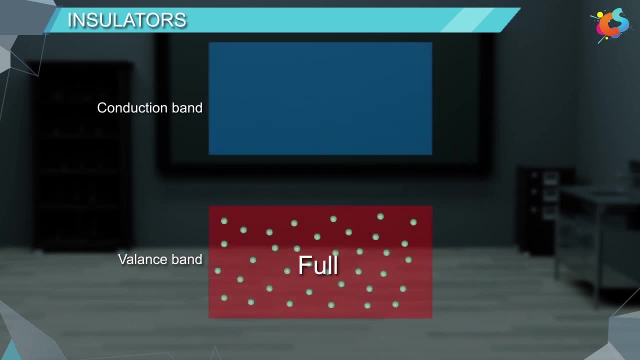 In these solids, the valence band is full, while the conduction band is empty. Even the forbidden energy gap between the valence and conduction band is large. As a result, huge amounts of valence can be found in non-metals. 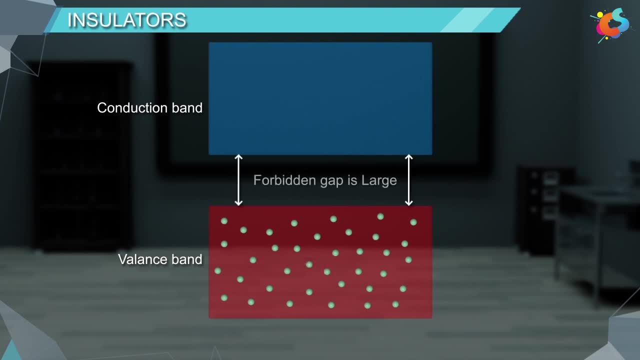 A large amount of valence can be found in a large amount of electric lights. In some cases the valence band cannot be filled. The valence band cannot be filled. The valence can be filled in one way or another. huge amount of energy is required to excite the electrons to the conduction band. Practically, 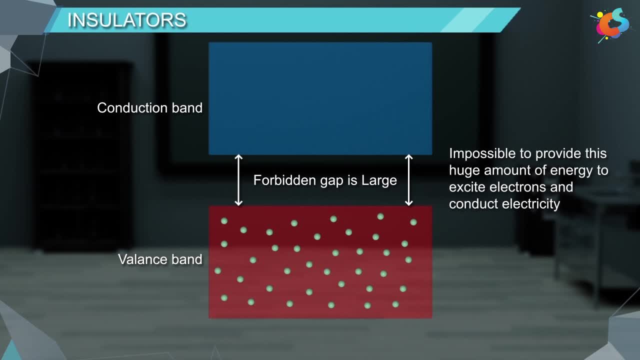 it is impossible to provide this huge amount of energy to excite electrons and conduct electricity. Therefore, most of the non-metals are insulators.